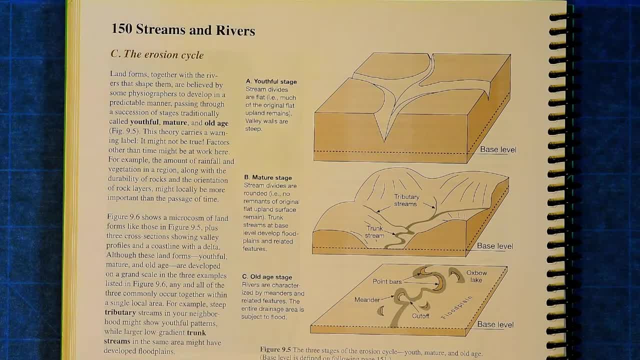 in question 9.6,. you are going to determine, looking at topographic maps, if a stream is in the youthful stage, mature stage or old age stage And the youthful stage. you're going to have lots of steep slopes, straight streams and narrow valleys. In the mature you're going to start. 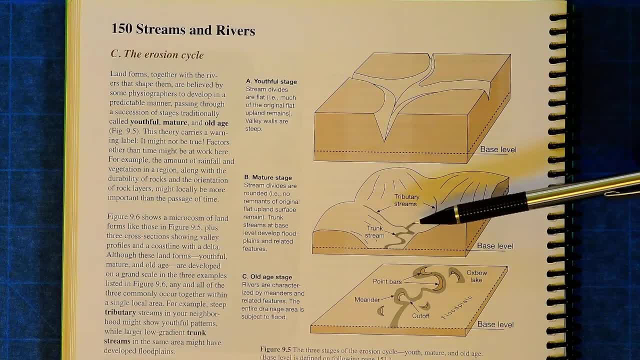 getting some curves in that stream and the topography is not going to be as steep And in the old age stage you're going to see a lot of meander loops and oxbows and things like that. So just look at the maps that you're given and estimate this. Again, please try not to overthink. 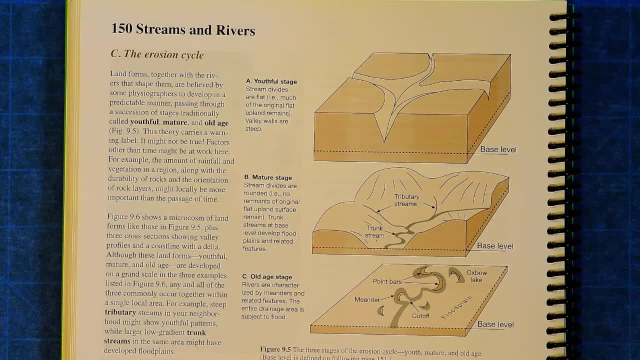 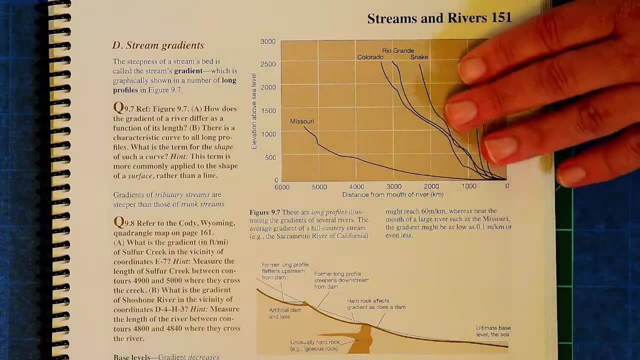 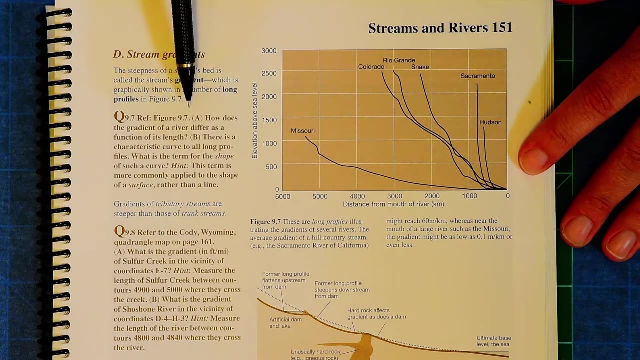 this too much. I think you'll be okay looking at those Other things to pay attention to in this lab. there's a question that uses this chart right here And it's question 9.7a and it says: how does the gradient of a river differ as a function of its? 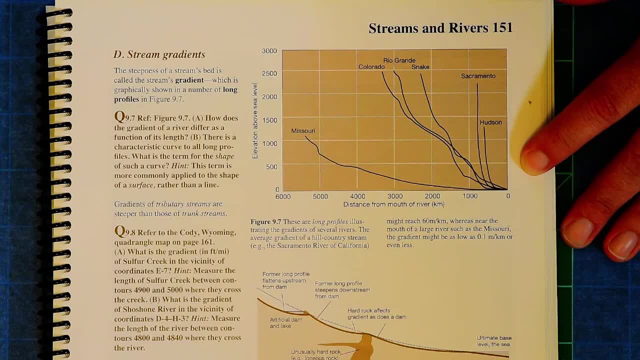 length. So what it's asking the gradient is the steepness of the river and it's asking how does the steepness change with length? And it's asking how does the steepness change with length? And what's plotted on here on the x-axis is the distance of the river. So the ones that are out. 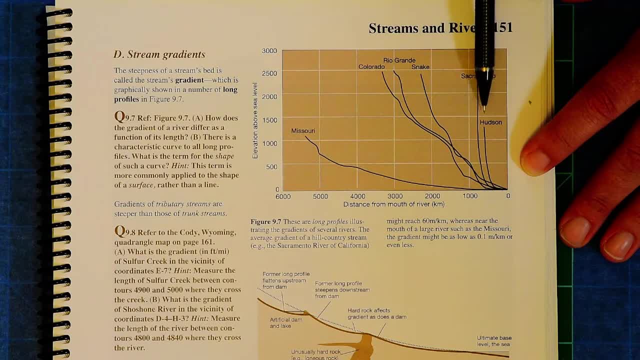 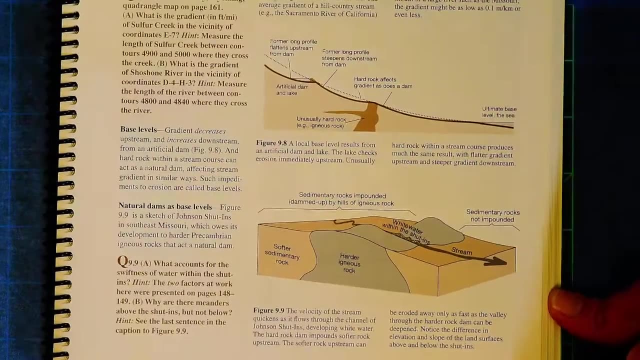 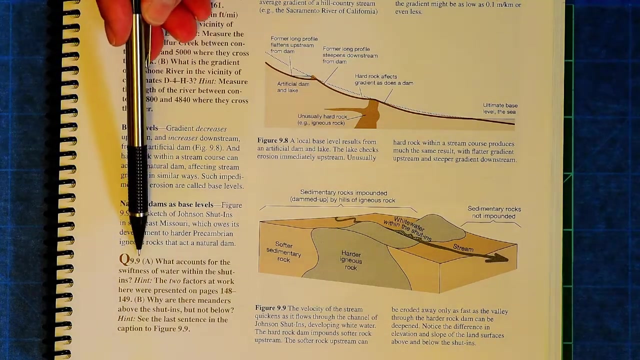 here. those are longer rivers. The ones that are here are shorter rivers, And think about how the steepness of that river changes as it gets longer. All right, other things right here. I can simply look down here. set the question 9.9,. it says what accounts for the. 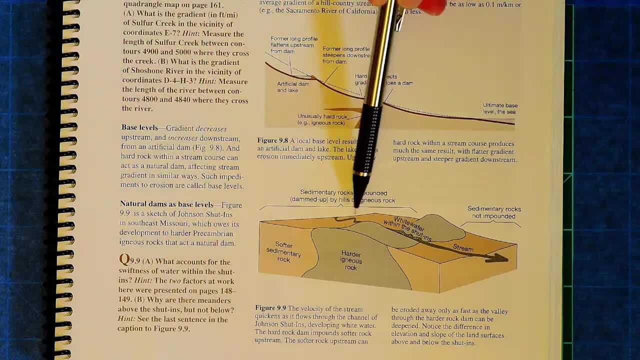 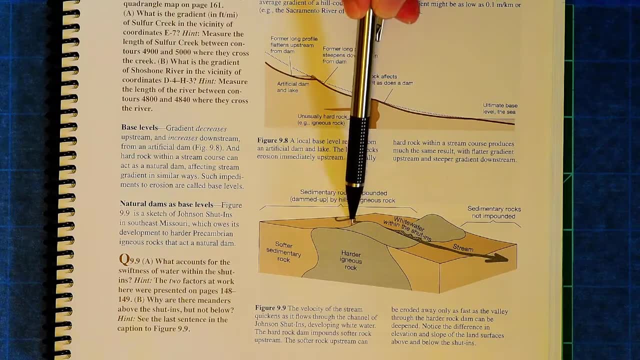 swiftness of water within the shut-ins. So there's this area where we have kind of this soft rock. here We have a meandering stream. It hits this harder. igneous rock races through that area. That's the area called the shut-ins. And then we have this area down here where the stream is stitchable. 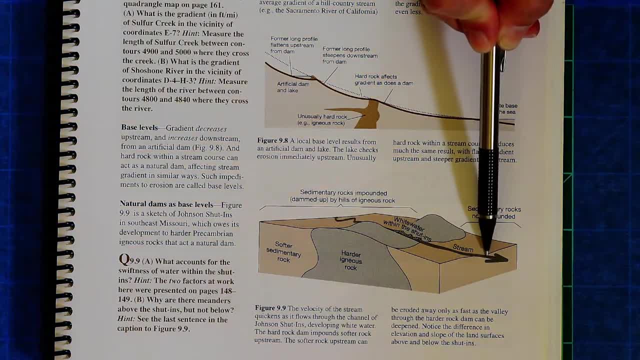 area called the shut-ins. And then we have this area down here where the streams are可是p种 and river doesn't absolutely slide. all the boxplay, it's basically pure lava up. have this area down here where the streams relatively straight, and so it's. 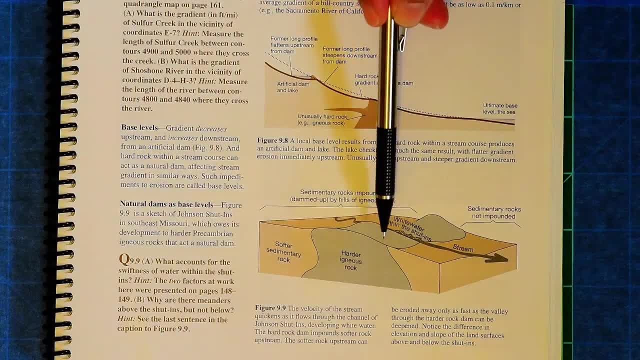 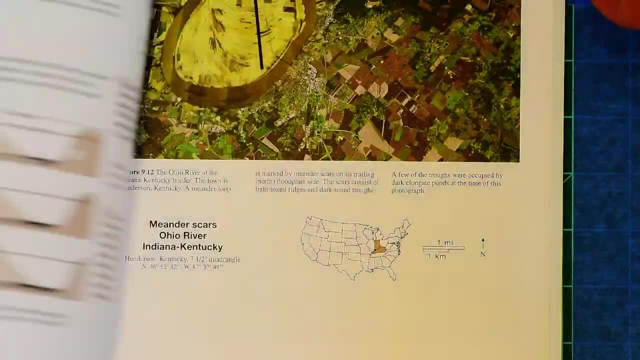 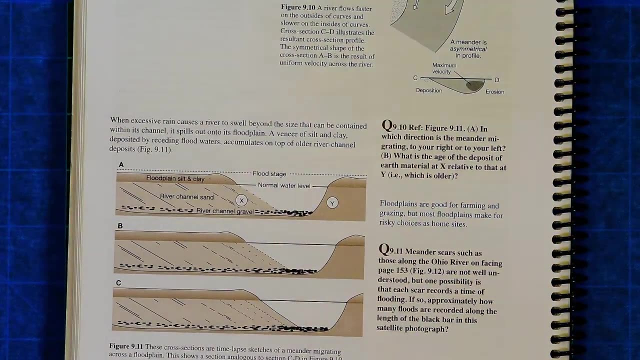 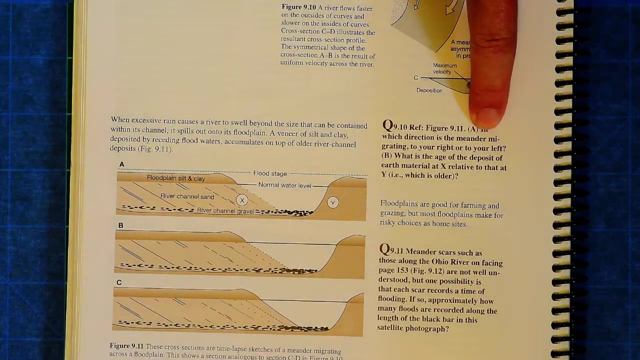 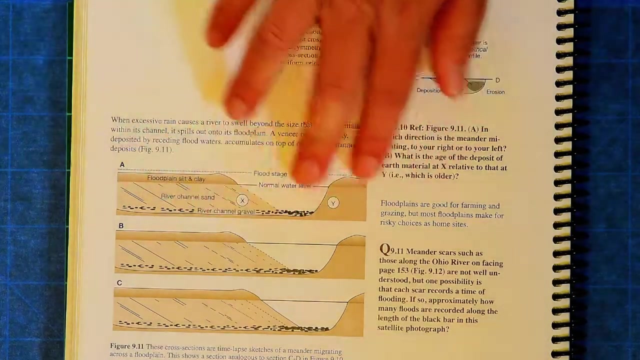 basically asking: what kind of characteristics would we have of the rocks here that make the water flow so much faster? okay, another question that you will be given in here. we're going to be looking at question 9.10. it says in which direction is the meander migrating- to your right or to your left? so we're 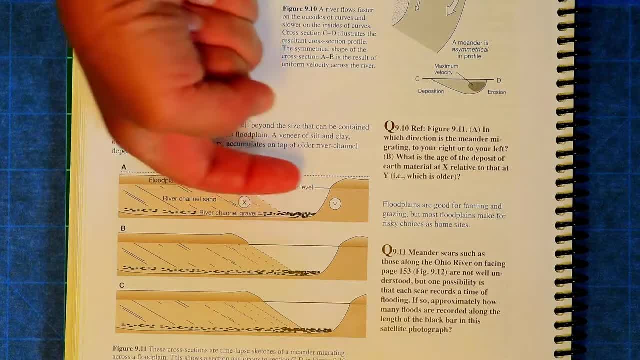 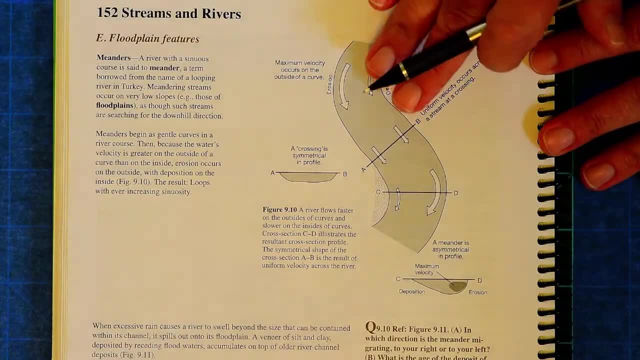 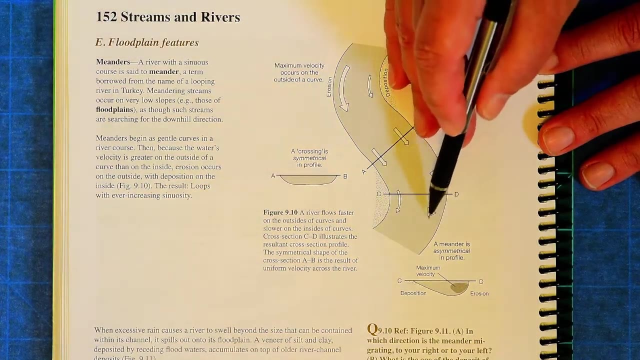 looking right here and seeing: does this meander, is the river eroding this way or is it eroding this way? so I just want to remind you: at these meandering streams, right at the outside of the curve, it's flowing fastest and you get erosion. the 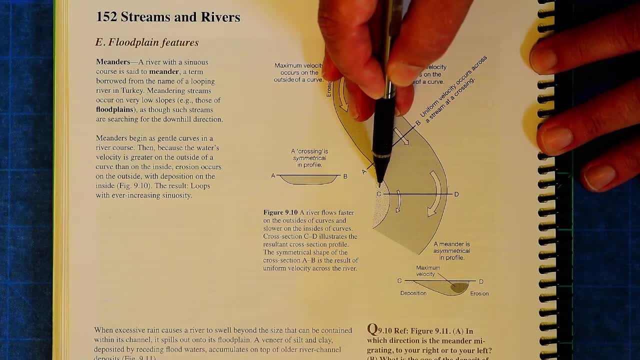 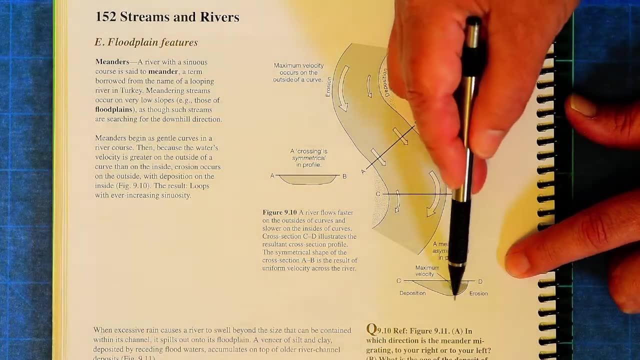 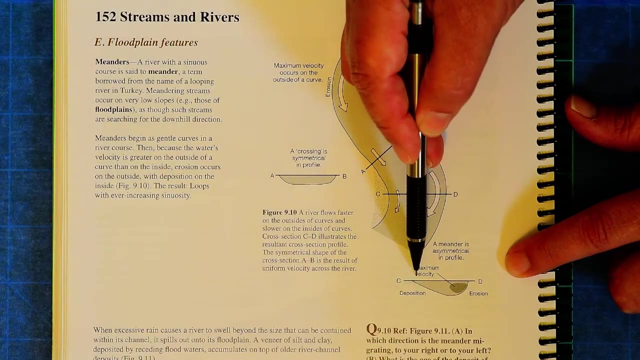 in side of the curve, it's flowing slower, you get deposition, and if we were to look at a cross-section, a side view of the river right here where we have erosion, that's also nice and deep. where we have deposition, there we have the shallower part of the stream. so now take what you saw there, look over here and 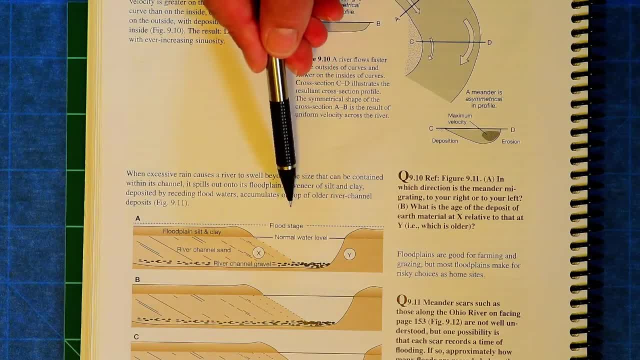 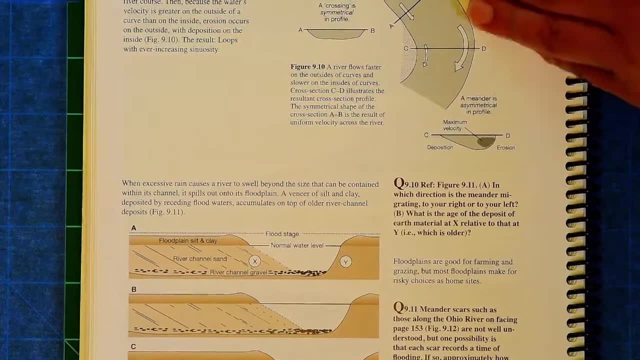 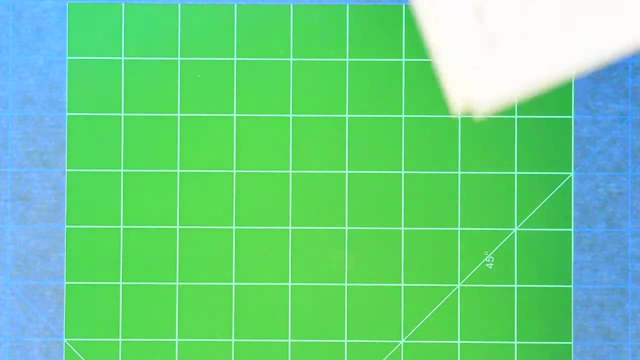 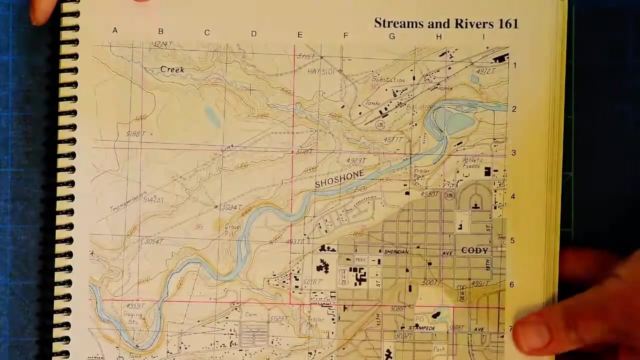 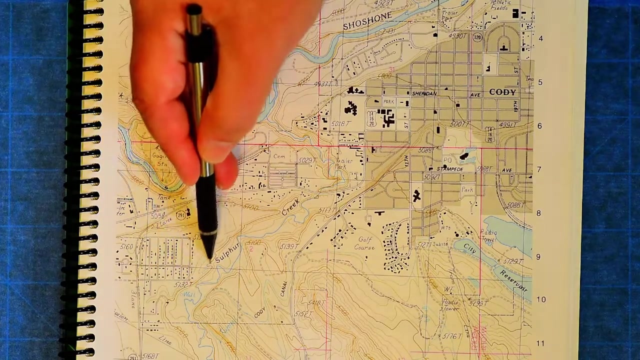 figure out where is erosion happening, where is deposition happening, and that should tell you in which direction the stream is migrating and let's see. last but not the least, let me find the right page here. you have a question somewhere along the line which asks if you are living along Sulphur Creek right here. you're living somewhere down. 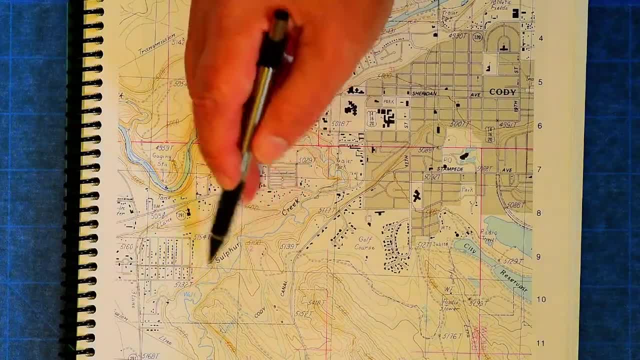 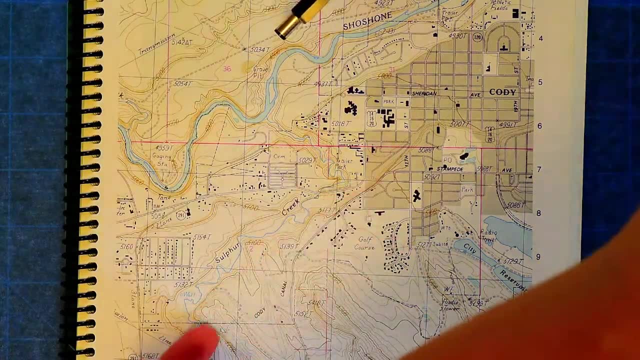 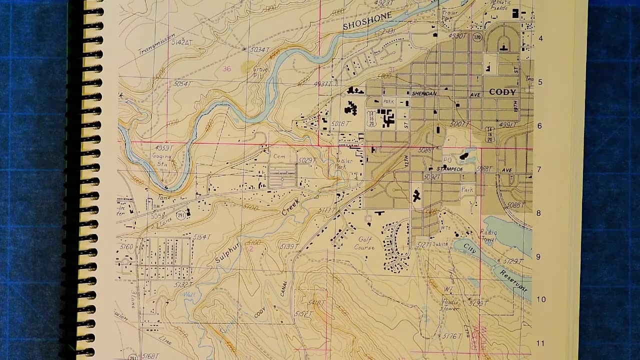 here and they decide to urbanize the area up here. should you be concerned, i would just like to let you know sulfur creek is flowing in this direction, so you are living downstream of the area that they want to pave over, so hopefully that will help you answer that question. as always, 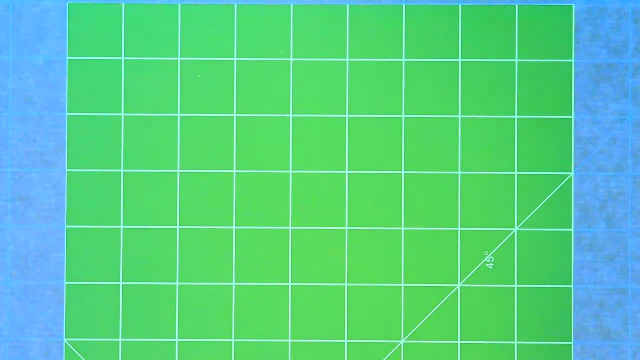 if you have any other questions, please let me know.